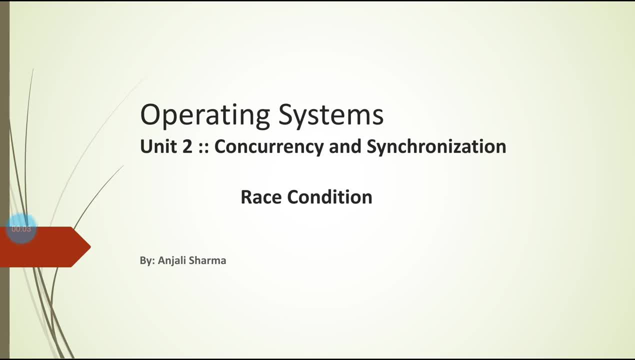 Hello everyone, welcome to operating systems lecture and today we are going to start our unit number two, that is, concurrency and synchronization, and this particular lecture will be devoted to the topic that is race condition, which is very important in terms of university examination. So let's see the timeline that what we are going to study today. 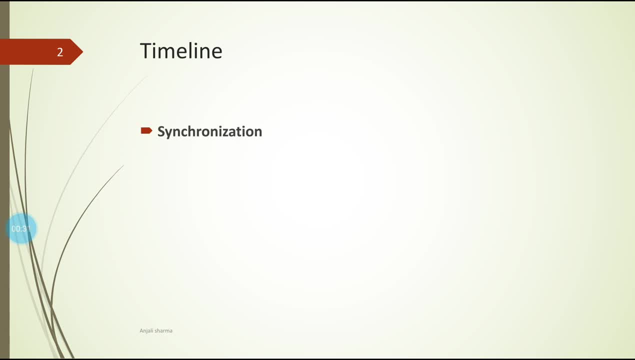 The first thing that we will be focusing on is synchronization. We will be seeing what synchronization is, why it is needed and how operating systems performs it. Then we will be looking at two different types of processes, that is, concurrent and independent. Then the race condition and, of course, the explanation of race condition with the help of an illustration. 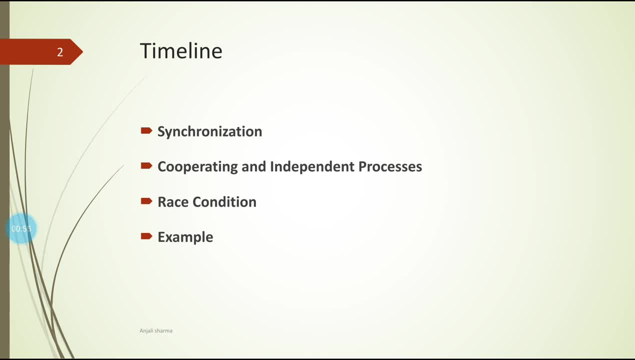 So, without much ado, let us start the lecture. So the main topic of this lecture is the question of race condition. The main topic to discuss about is: what do we understand by synchronization? and, to be very precise, it is the very important and considered as the heart and soul of your complete operating. 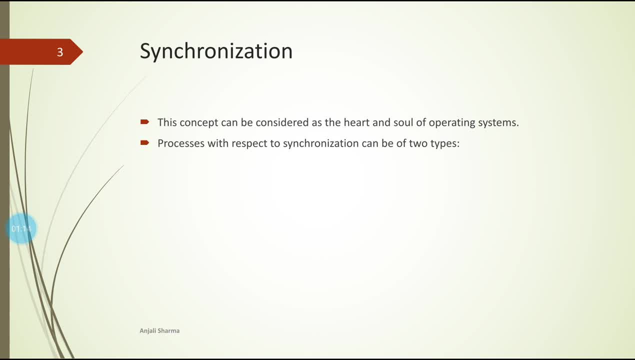 systems performance. See. the modern operating systems are either multi-programming or, we can say, time sharing in nature. That means that at particular time of analysis the main memory will be having a lot of processes in it, as per the degree of multi-programming. So the 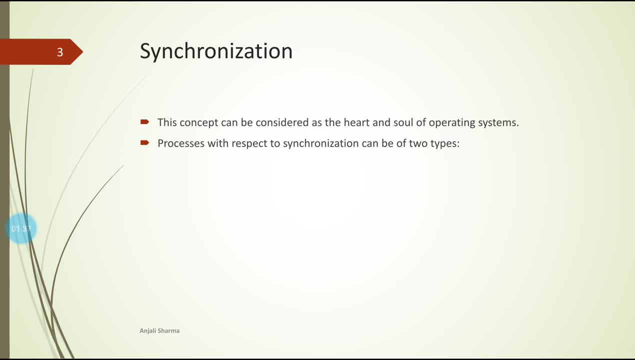 synchronization is very necessary among these processes so that the processor or CPU can execute these processes in an efficient manner. So, because of the multi-programming nature of our operating system, the concept of synchronization came into view. So we also know that that there are different types of processes in our memory or in our computer system as a whole. but considering 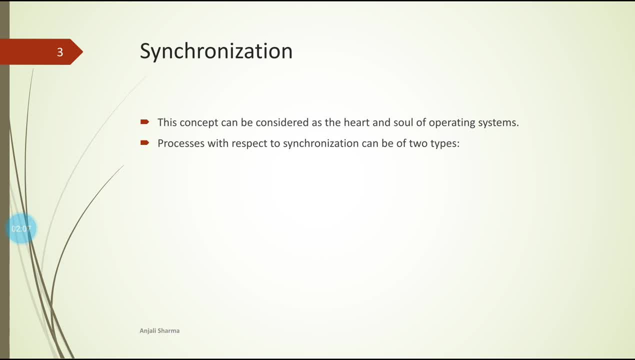 the topic of synchronization, the processes can be divided into two types. According to synchronization, processes can be either cooperating or independent in nature, And it is to be noted that if the processes are cooperating in nature, they require synchronization, whereas if the processes are independent, then they do not require synchronization. So the coordination among the processes or the 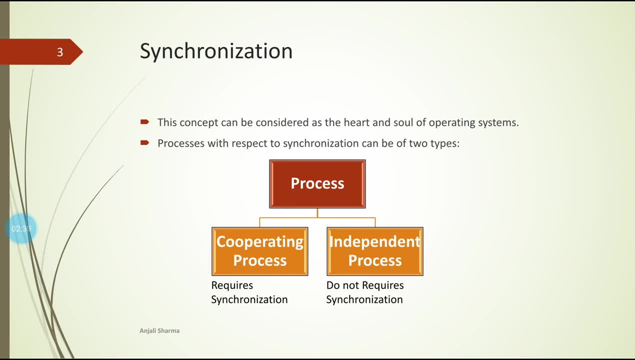 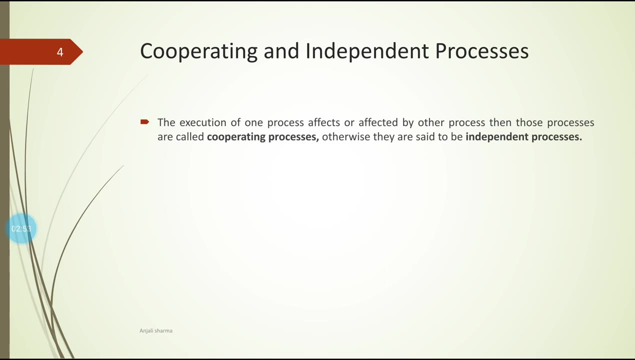 synchronization is performed when the processes are cooperating in nature. So now let us see what we exactly mean when we say that this particular processes are independent and other are cooperating. So the definition of cooperating processes says that when the execution of one process affects or is affected by other processes, then that is termed as a cooperating process. 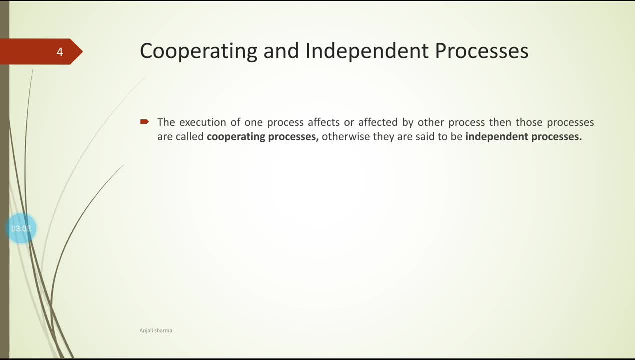 otherwise they are independent. So let us understand it with the help of an illustration. Suppose we have two processes, process 1 and 2, and they are manipulating a single shared variable. Process P1 is adding 10 to x, while process P2 is subtracting 10 to x. 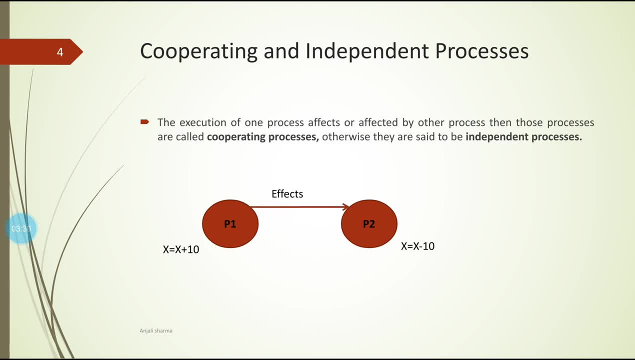 And now suppose that if process P1 affects the process P2 somehow- or we can say the other way around- that process P2 is affected by P1, then they are termed as cooperating. Now, this affecting or affected by nature is because these processes will be interacting to each other during their 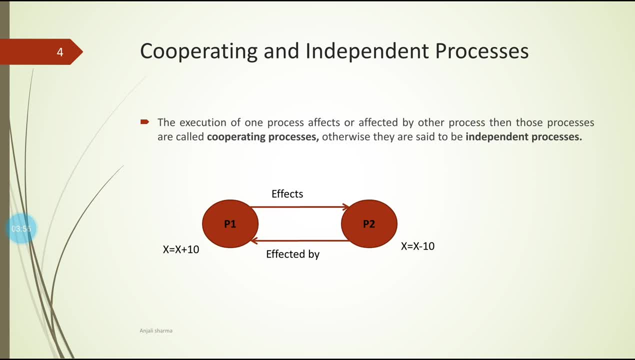 lifetime. They are indulged in an inter-processed interaction, So the process P1 is affecting the process P2 and the whole process P2 is an inter-processed interaction. So the process P2 is a miscommunication that can be performed either by shared memory or by exchanging messages. 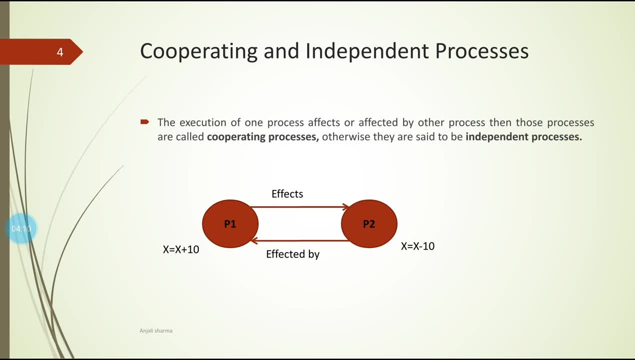 Another thing that if these two processes do not interact with each other at all during their lifetime, then they will be termed as independent, and remember that independent processes do not require to be synchronized. Another point that is to be considered when the processes are cooperating is that that this affecting process can be involved in any type of inter-processing. 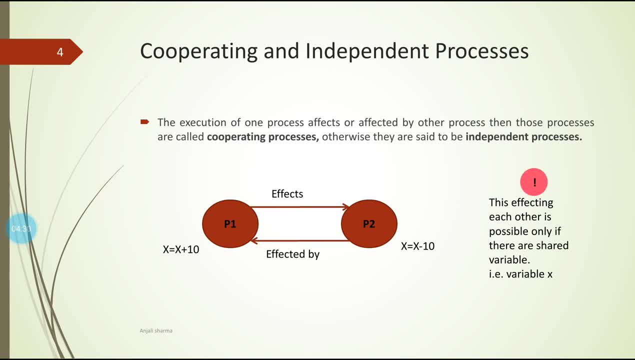 or inter-processing. So in this case the process P1 is just acting as the inter-processor, So the process P2 is each other is possible only if there are shared variable, and in this particular case, these both processes are manipulating on a shared variable, x. so whenever the cooperating processes are sharing, 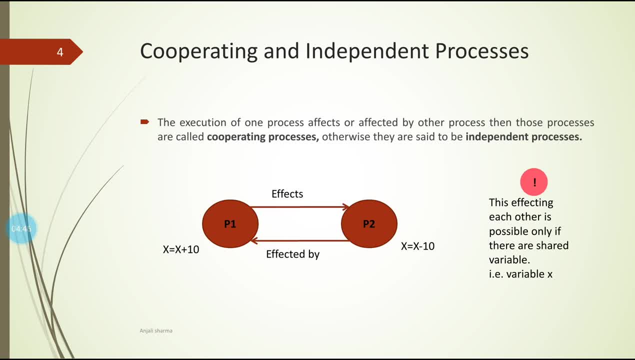 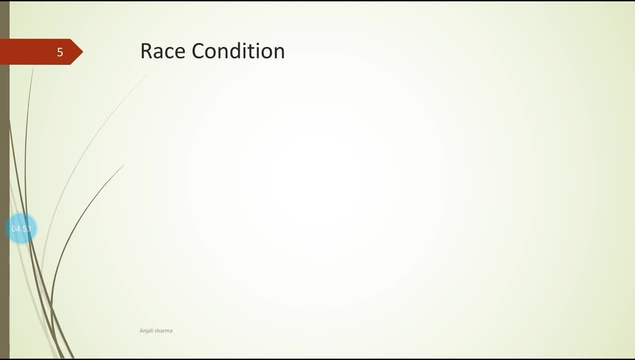 the common data structures, variables, files or table, then there is a need of synchronization. so this synchronization problem give rise to an inconsistency among the system which is known as race condition, and the complete unit. 2 will be revolving around the solutions to remove race condition from our cooperating processes. so let us see what do we understand by race condition? 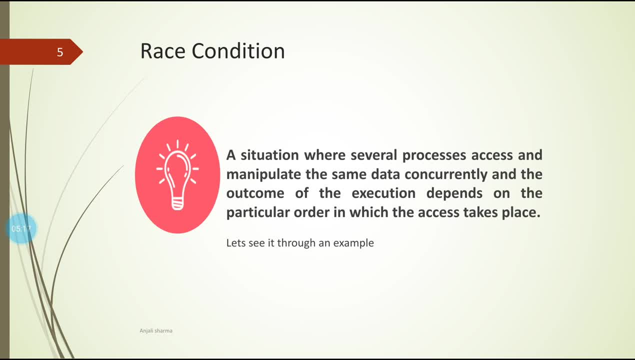 it is a situation where several processes access and manipulate the same data concurrently, and the outcome of the execution depends upon the particular order in which the axis takes place. so if now the definition is feeling something overwhelming, let us understand it with the help of an example, because illustrations makes things easier to understand. what does it mean that the 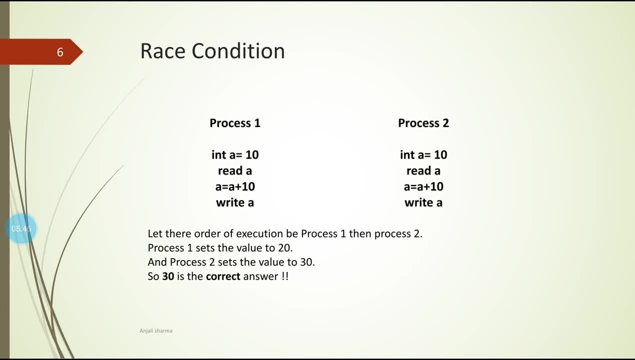 race condition will arise in a cooperating process. let us see, suppose we have two different processes. processes p1, that is, having a variable a equals to 10, it reads its value, add 10 to it and then write it value in a variable a. again The same code is copied in the process number 2, it also reads: 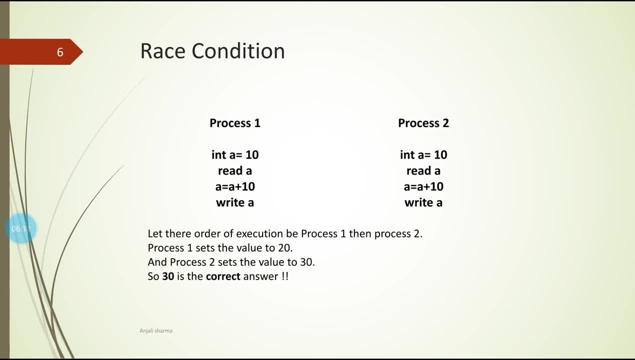 the global variable a as 10,. it reads its value, add 10 to it and then write it. Now let us order the execution of these processes. The process 1 will be executed first, followed by the process number 2.. So the process 1 will set the value of a as 20.. Now the a is changed to 20 and after that 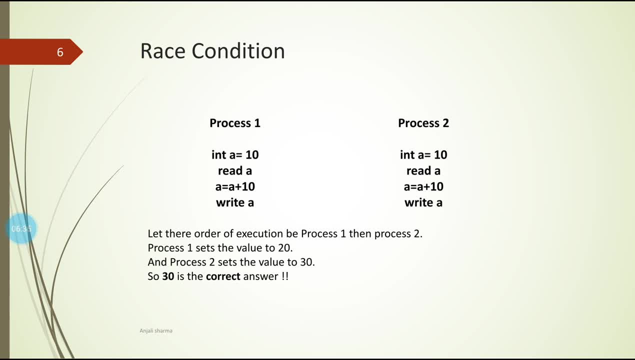 process. p2 will be executing its code, So it will again reading the value of a as 20, add 10 to it and write 30 into the variable, So the correct answer will be 30.. In this particular situation, remember, the logical correctness of a cooperating process depends. 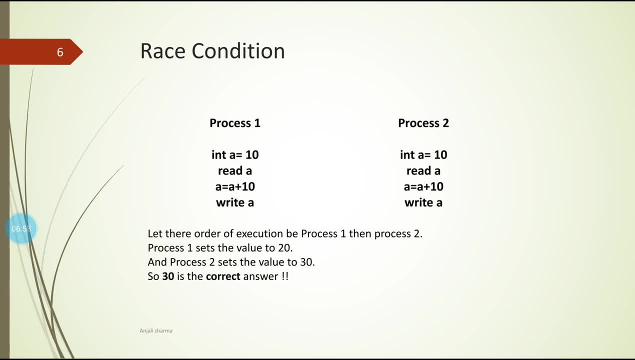 when their order of execution is followed strictly. So the correct answer will depend not only on the logical correctness, but also the order of their execution. But we need to understand that we are working in a multi-programming and a time-sharing environment. Let us consider: 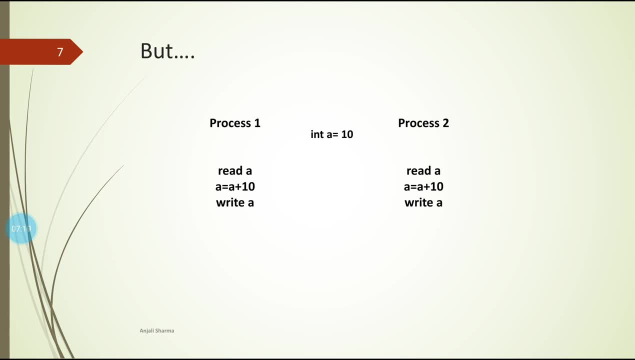 this particular scenario and we will see how inconsistency arise because of race condition. So again we have these two processes: a global variable a and the both processes are adding 10 to this variable and writing its value. Suppose this is a GAN chart which will be showing: 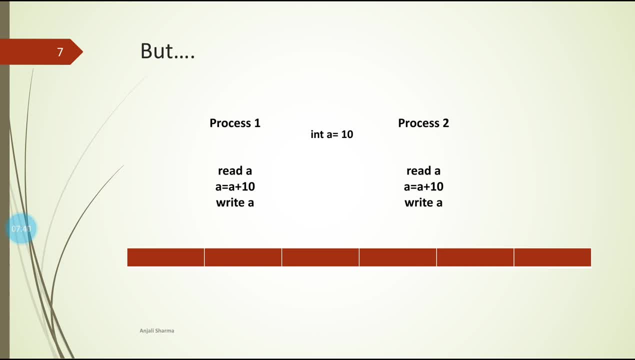 the proper execution of the processes. Now, as per the algorithm, suppose we are using ground robbing for the scheduling of these two processes. Process p1 comes into the CPU, it gets executed and it reads the value of variable a as 10.. Now suppose its time quantum gets expired and the process p1, that 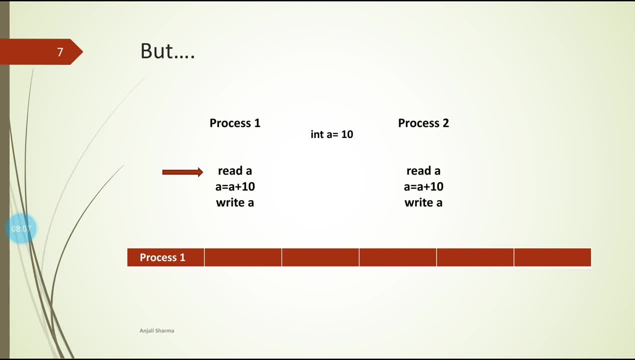 is, the process 1, which is now currently been executed by the CPU, will be removed from it temporarily to the waiting queue. then the process p2 will also be executed and also its variable A will be removed from the CPU, and so on. And so let us see with site through the all layers menu of GAN: permite la vista e here il境 qucemium ainto in the process d' Гl nied醒 c de process p1 der SCOTTES P1 M switch ii e na melentice dem lexii. 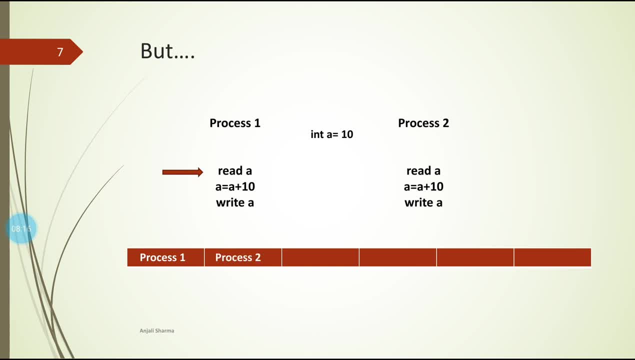 denLike this, the process P2 will get the chance for execution and it reads the instruction, read A and gets the value of A as 10.. Suppose again the time quantum expires and process P1 again gets back the CPU. In this particular point of time it will be executing its next instruction, adding 10 to. 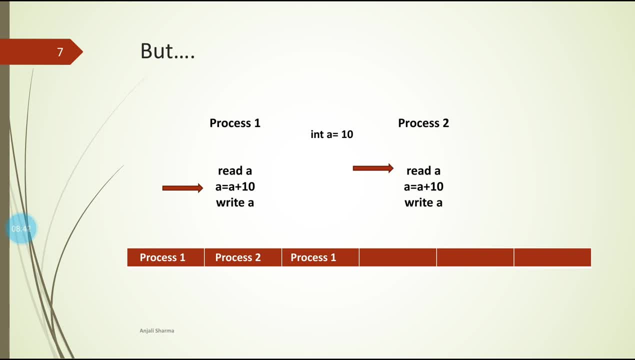 the variable. Again, context switch occurs because the time quantum gets expired, Process P2 will regain the CPU and it will be again adding 10 to the variable A, which it has read as 10.. So the value of A will also becomes 20 for process P2.. Again, context switch happens. P1 regains the CPU. 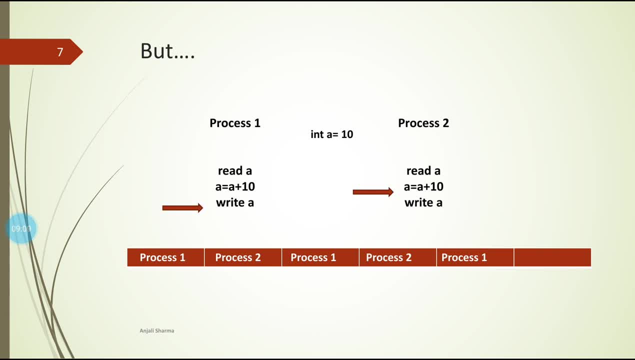 and it will be writing the value of 10 to the variable A As 20.. Context switch happens Again. process P2 will regain the CPU and it will be again writing the value of A as 20.. But in the previous slide we have seen that as per the order of execution.